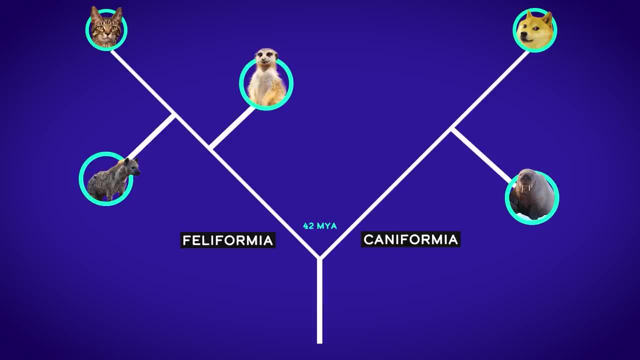 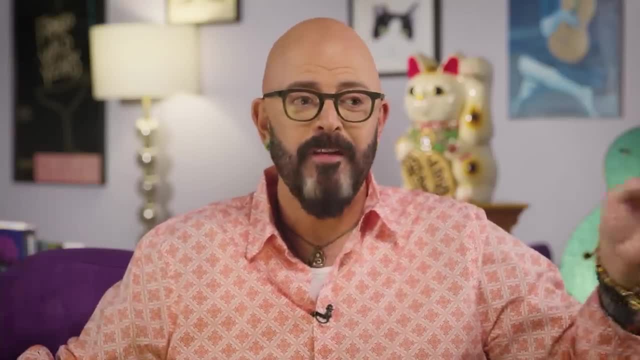 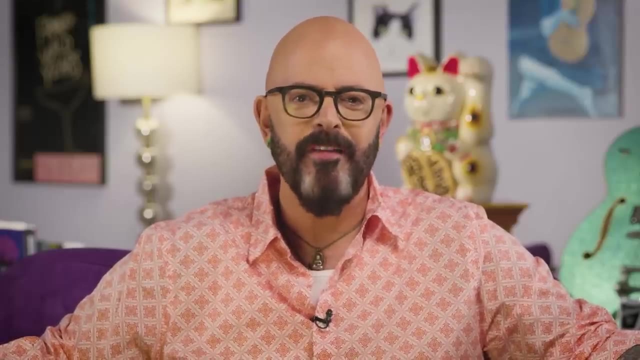 in the the caniform. I mean just saying that blows my mind, let alone trying to come up with the, the plural for mongoose and walrus, because they're not walri, nor are they walruses. walri, walri anyhow. that is just not part of this video. so, with the mind-blowing facts aside, we're 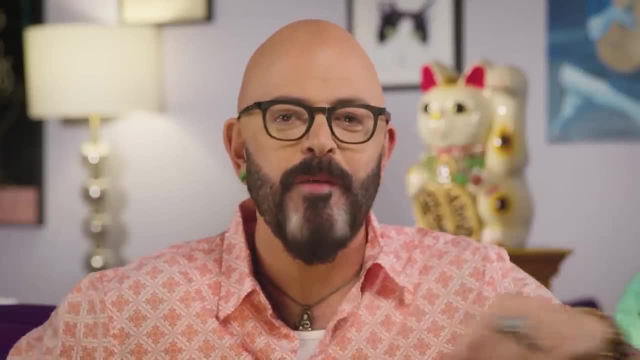 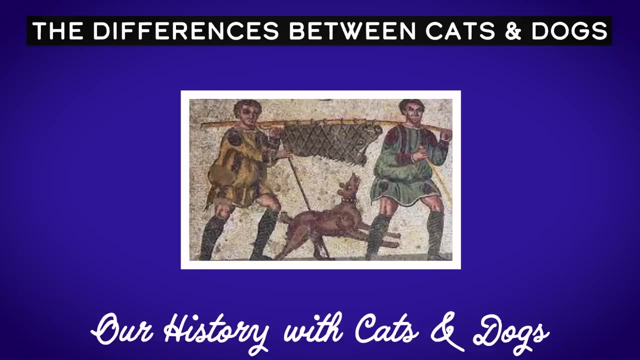 still making a video because everyone's still asking: what are the main differences between cats and dogs other than the fact that a dog is not a walrus and a cat is not a mongoose? so let's get into it. it really does come down to this evolutionary difference. that's really the. 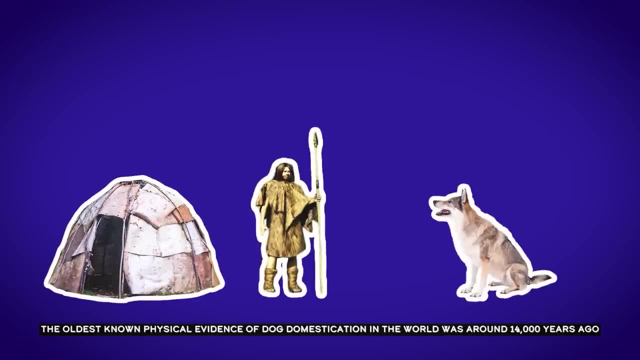 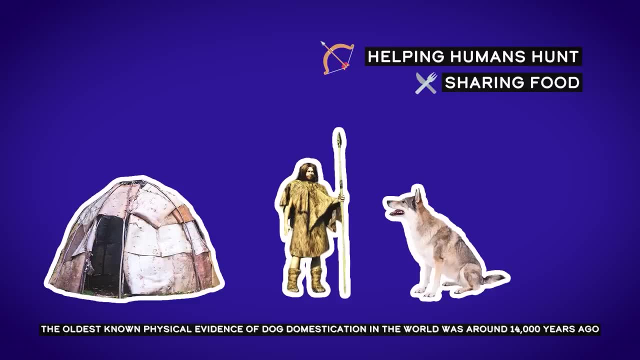 journey of domestication with dogs. we co-evolved with them from that time. they came in with us and it was all about helping us hunt, sharing our food and then, you know, striking this bond and, over time, selectively breeding them to do very specific jobs, and we're still making a video about that. 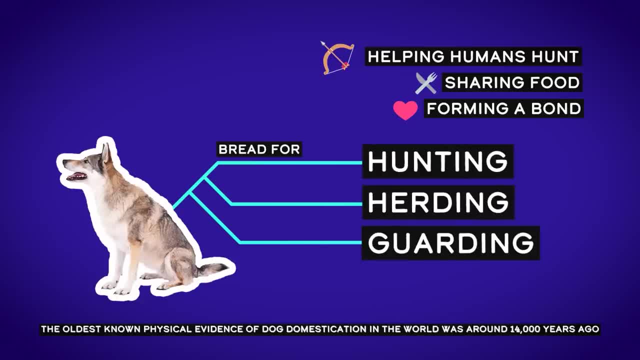 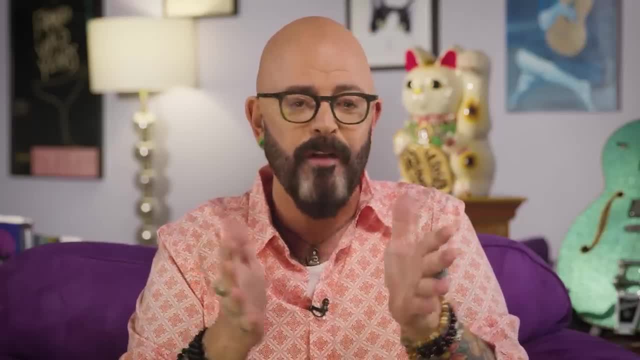 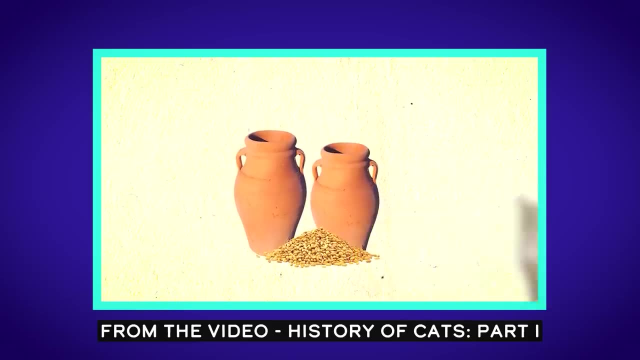 and in the meantime they became companions. and that is the long history with dogs, with cats. it really came down to this mutually beneficial relationship, starting 12 000 years ago, where we were storing grain, the, the mice and the rats were fouling that grain. the cats came along, took 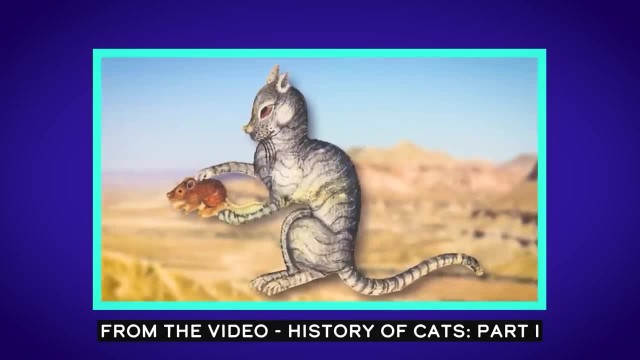 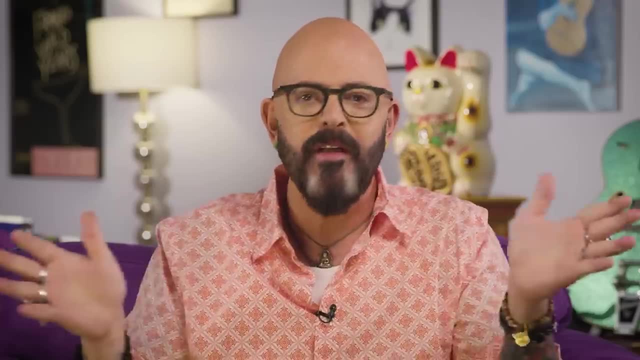 care of the mice and the rats, we said, well, this is a great relationship. when it came to calling them companions. really, that's a blip in the timeline. we're talking about a couple of hundred years, as opposed to a couple of years ago. we're talking about a couple of hundred years. 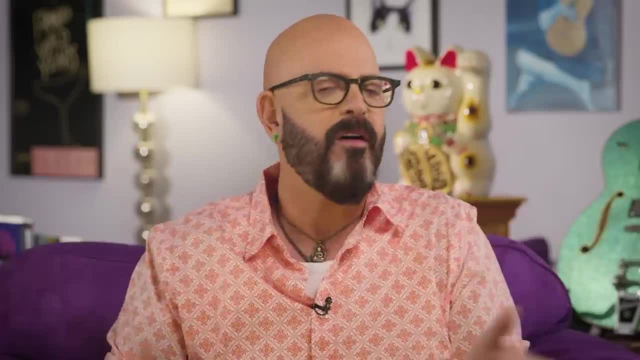 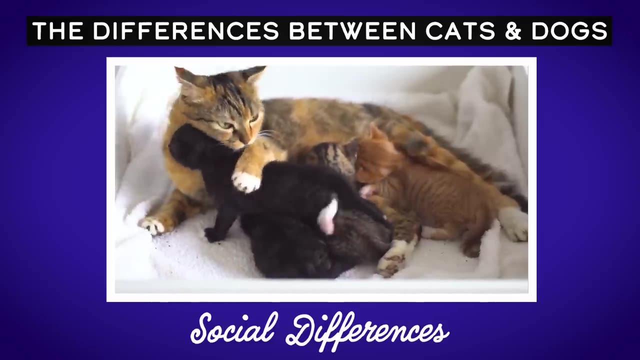 ago. we're talking about a couple of hundred years ago. we're talking about a couple of hundred years, the 40 000 years with dogs, and as we start talking about all the rest of this, you'll see it all flows through those very basic facts. so now we start looking at the big social difference between cats. 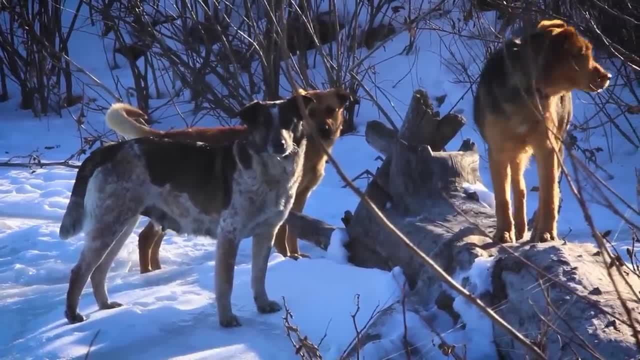 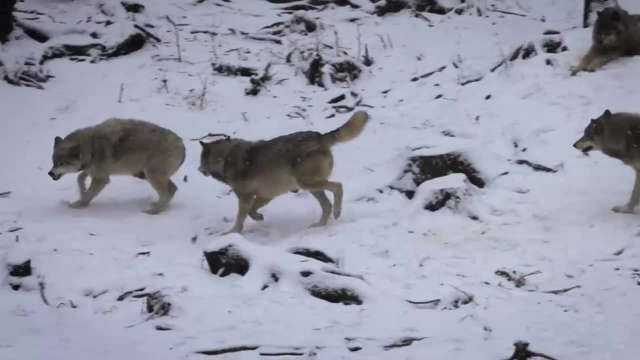 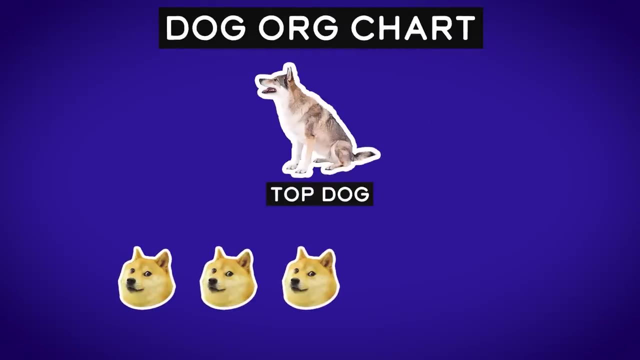 and dogs. there has been a rift as to whether we see them as pack animals because the wolves were pack animals, but we're a long ways removed from that and really do dogs see each other in this very strict step step system like alpha dog? but let's be general about this. dogs have a much more. 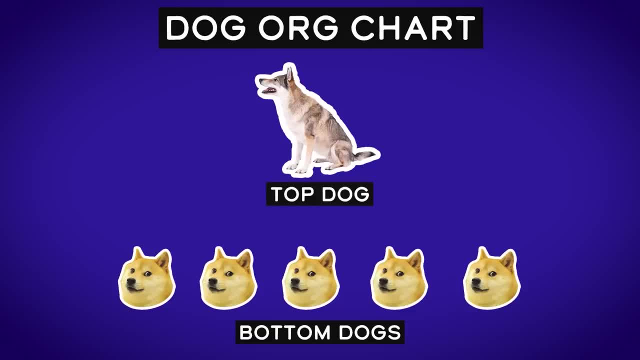 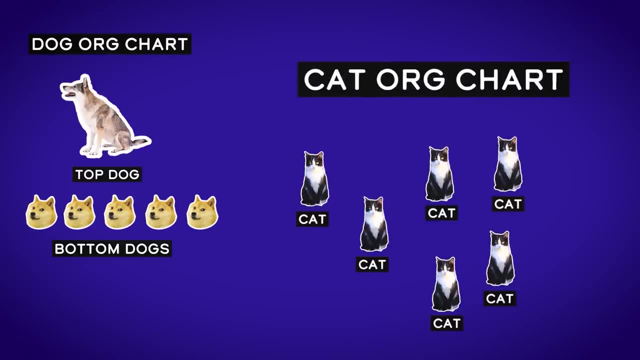 rigid way of seeing each other, and that's what we're going to talk about today. we're going to talk about this dog as a society, as a group, whether that be pack or not, then then cats do, because really cats do not have that strict hierarchy. they really don't. in fact, if you look, 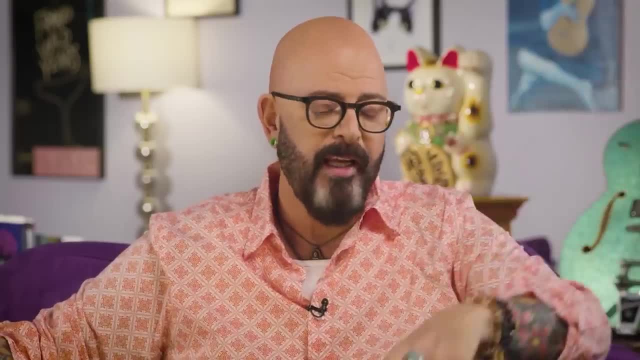 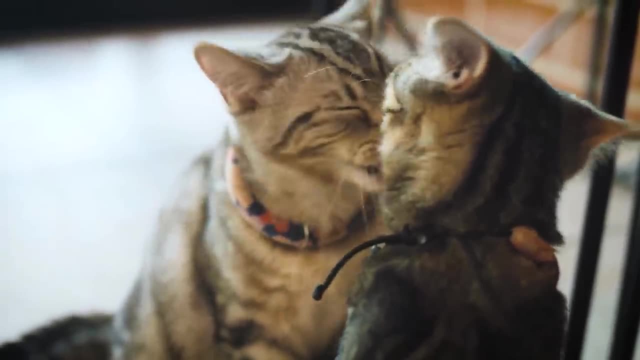 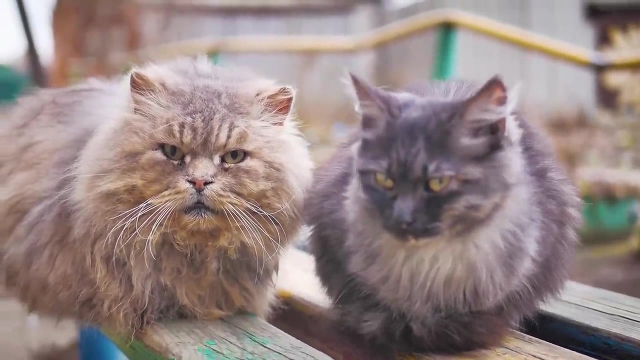 at cats in in colonies outside. if you look at them as in a social way inside, there's much more that we don't know about cats than what we do, and that's the truth. i mean, for every study that has been done about this, there's 10 that need to be done, or we may never know, but we do know that cats 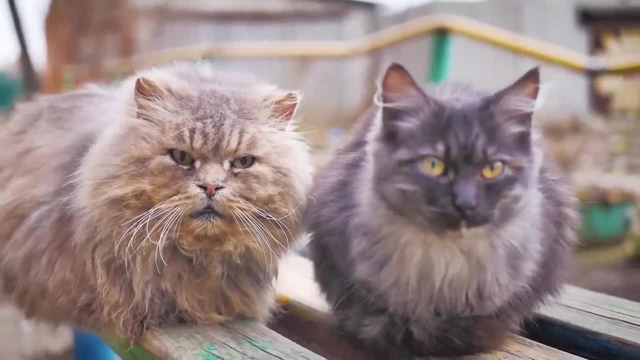 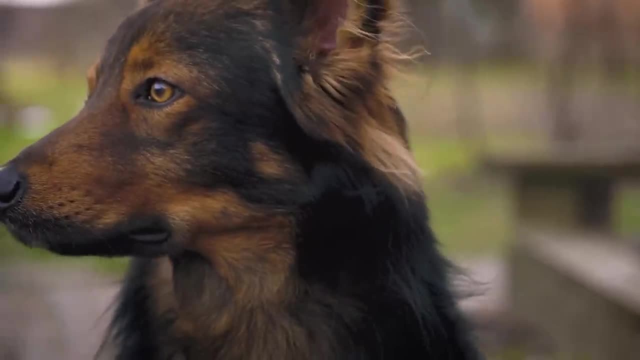 know how to live in a society where cats are not as social as they are. in a society where cats are in a community. it's just much more in flux when it comes to the way that dogs see humans that they really look to us for their cues and for their well-being. cats not so much because, again, we've 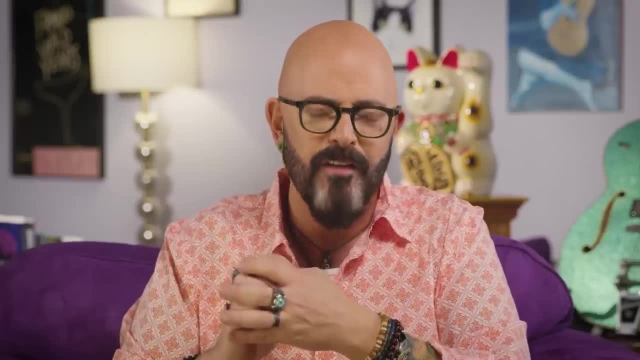 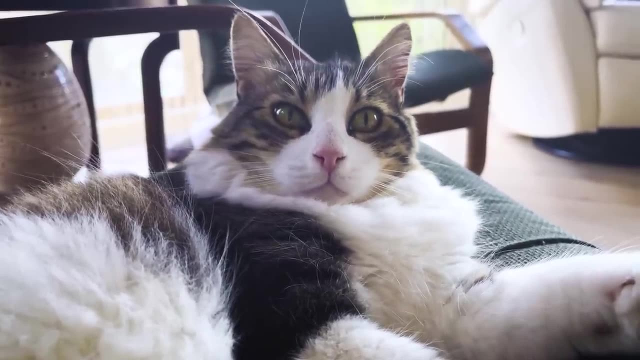 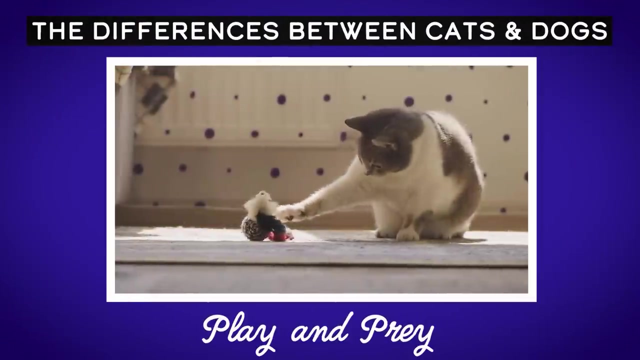 just really been in the same home with them for not such a long time. cats still retain a lot of that wild, but that is not to say that they are not sociable and social with us. it's just not the way it is with dogs and that is a big difference between cats and dogs. and not to belabor the 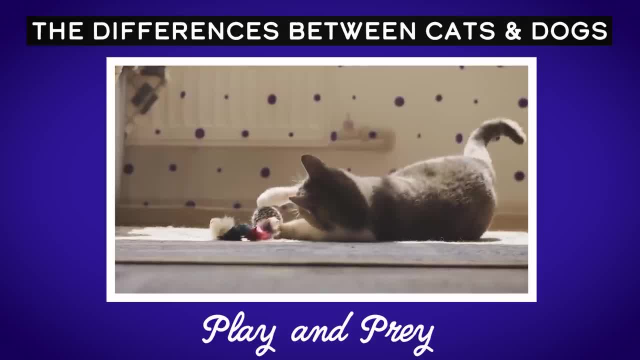 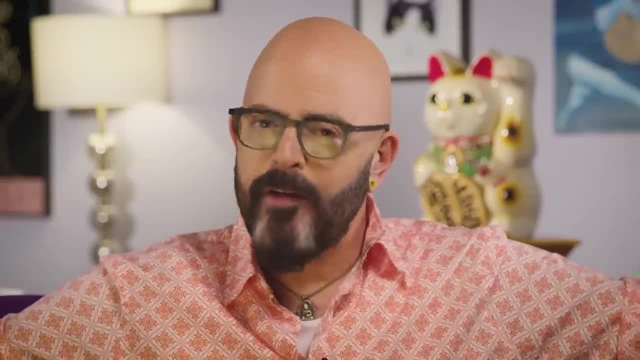 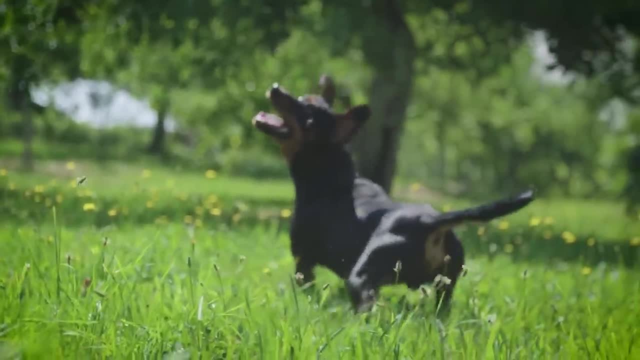 point. but everything i talk about here is all about the straight line between who i call the raw cat, the ancestor, and your cat. it's a very straight line. all of the behavioral characteristics- and social and physical- all relates straight back there. so with playing with a dog they can go for. 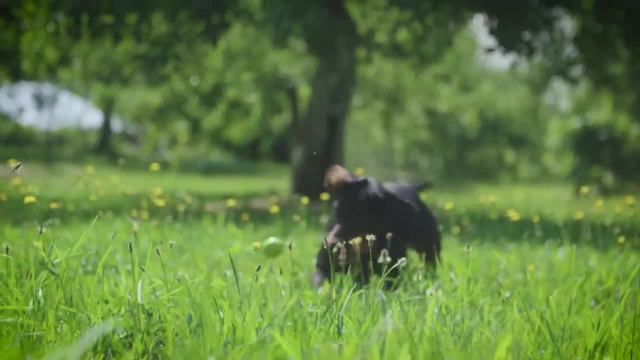 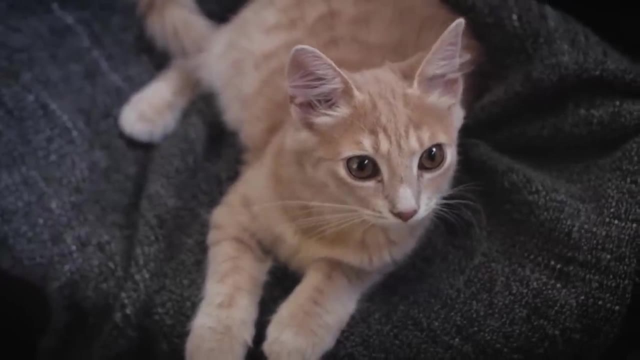 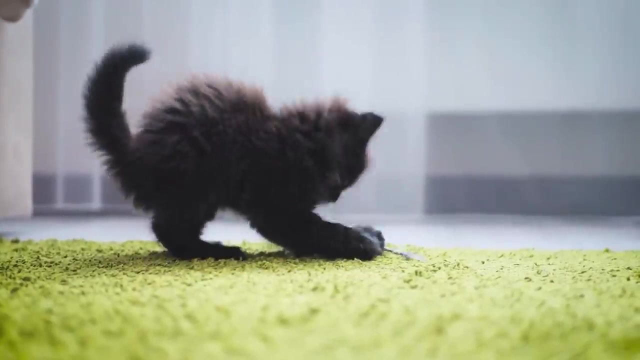 like an hour. anybody who plays with dog knows that that the fetch can go on for an hour. the running around can go on for an hour. with cats it is just not the case. cats are built for speed and not play equals prey. from a very, very early age this is what they know. hunting is play, so a cat as a 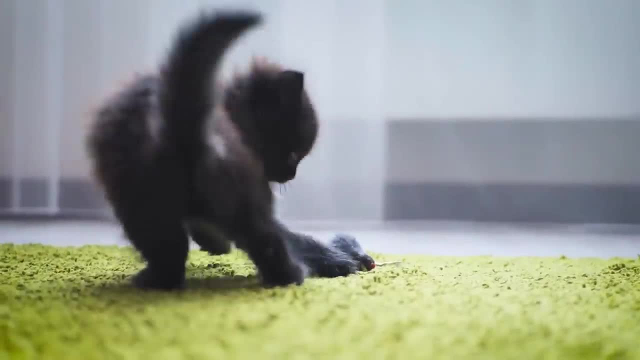 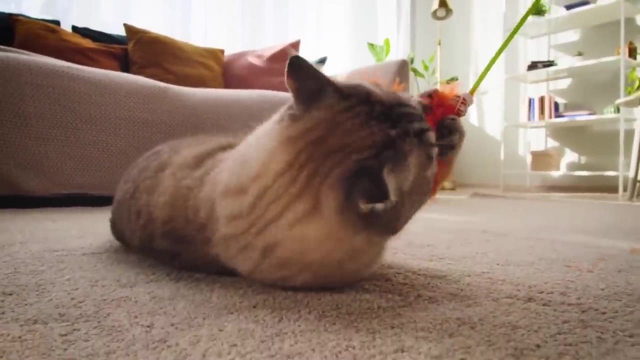 hunter is meant to: to watch, to assess, to stalk, to pounce. if they don't get what they're after, they go right back to square one and do it again. so it's very short spurts of play and i think again, as we expect cats to play, we think they're going to play like dogs and we're disappointed when they 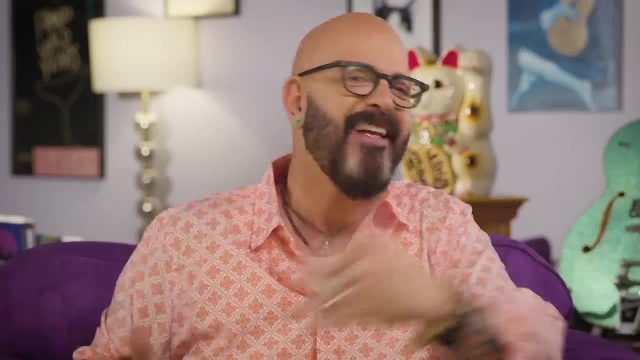 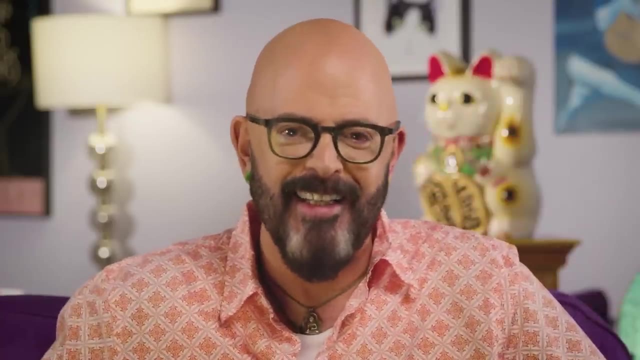 don't run around for an hour and that's not who they are, and everything i'm going to say from now on is the same point. so you can rewind the video and go right back to the beginning of the video if you're trying to figure out some context physically, so let's talk about the physical. 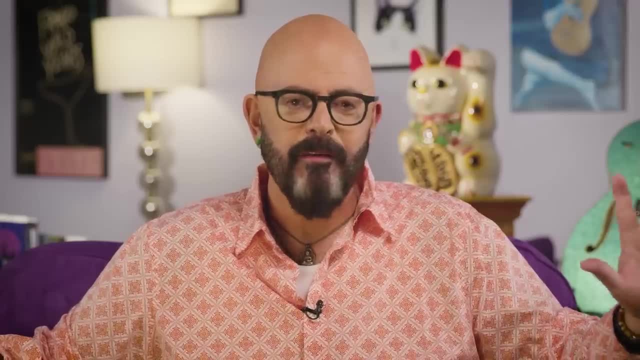 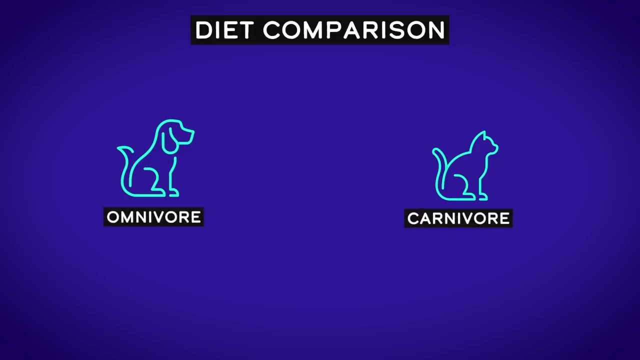 differences between cats and dogs. i want to start right at at the, the center of everyone's lives, which is dietary needs. dogs are omnivores. now, yes, both cats and dogs evolved as scavengers. that's a similarity. but dogs were scavengers but also depended on what we were eating. at the same time, 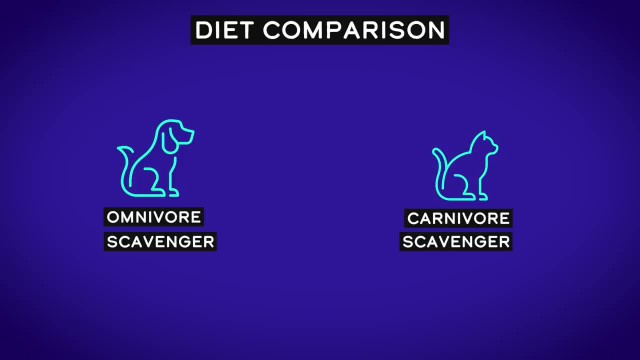 and that's why dogs can be more carnivorous. they can be vegetarian, they can be vegan. they can live on any of that sustenance- cats can't. the difference there is that cats are obligate carnivores again. we haven't done much to their process over all these years. they still need what they needed. 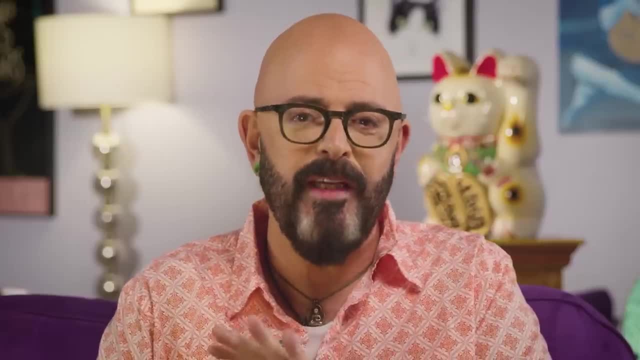 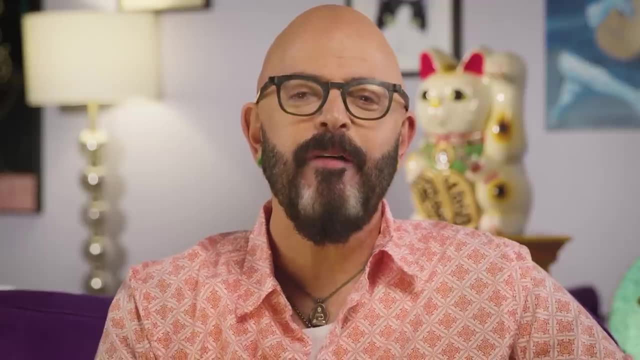 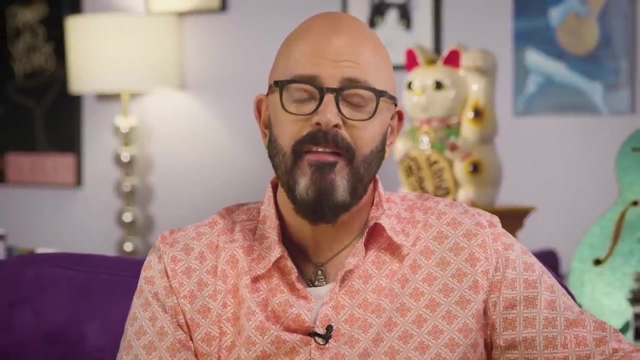 tens of thousands of years ago. that's why cats cannot be vegetarian, they cannot be vegan. they are obligate carnivores. you know what allows me to make videos for you guys on an ongoing basis? 350 videos and counting. that is your subscribers. a lot of you guys think you're subscribed, but you're not as a matter of fact. 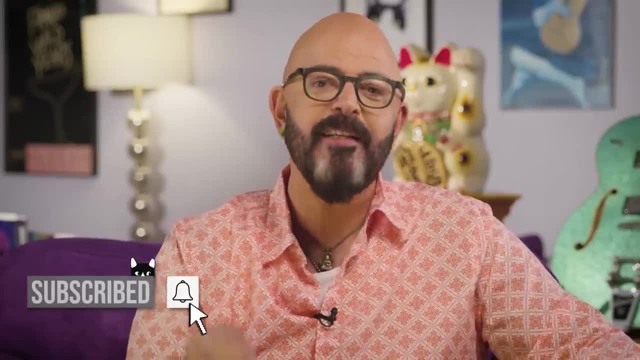 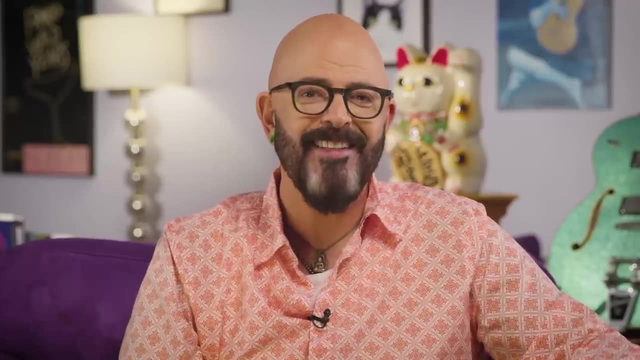 over 70 of you who watch these videos are not subscribed, so please subscribe. hit the bell so that you know when videos are coming out and also what helps our channel is like. so do that too. another big difference between cats and dogs is their feet. i know some of this sounds a little. 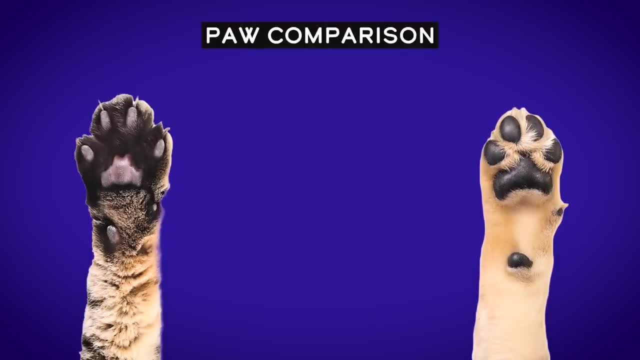 obvious, but not so much now. a similarity is that both dogs and cats cool themselves, uh, through their pads in their feet. they basically sweat through their pads. another big difference- in their feet dogs have nails, cats have claws, and again that's a big difference- is that the claw is just a really basic part of a cat's life as a solitary hunter. 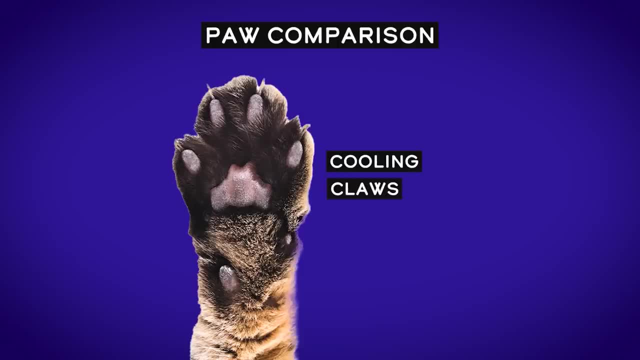 as as someone who's in nature, right in the middle of the food chain, hunt, be hunted, kill or be killed. those claws are really important. it is a offensive weapon, it is a defensive weapon and this is a very big difference between cats and dogs. dogs are, by and large, terrestrial. cats own the sky, and that's the thing. cats vantage point, escape routes. 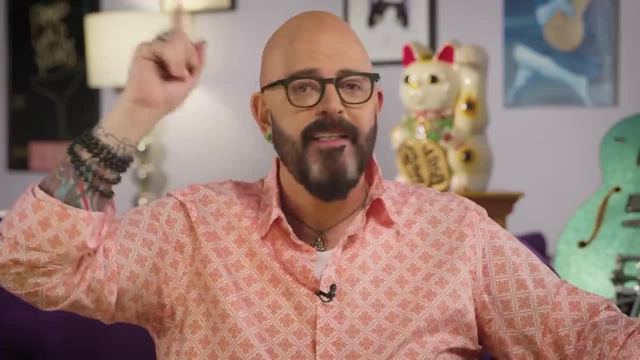 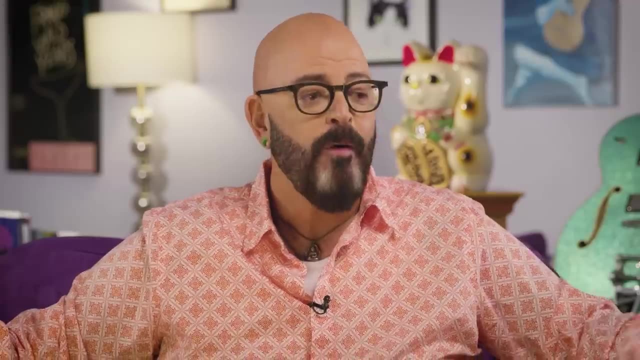 you know where they are the most confident in the world. oftentimes it's up there, and any of you guys who have cats know that. because we talk about catification, environmental enrichment, and when we talk about that, we talk about them not having to share the space with dogs and to create their 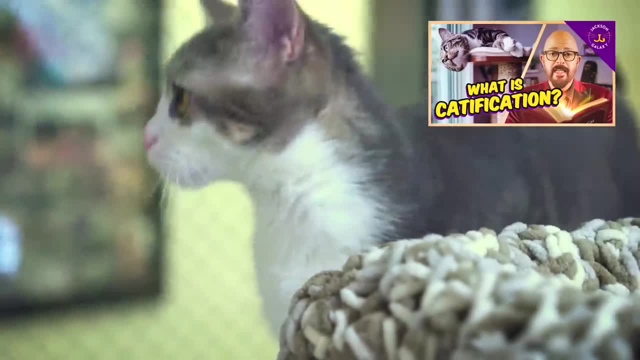 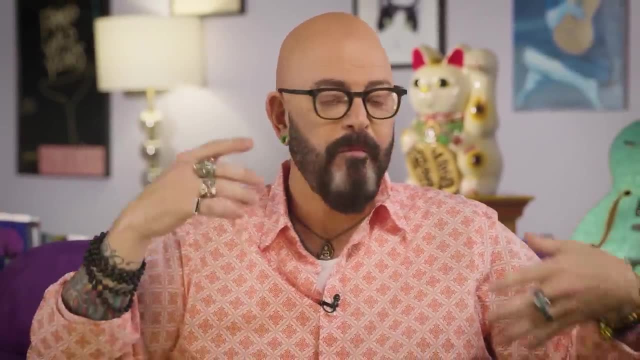 own lanes of highway, which often is going to be off the ground, and so much of that is about their claws and an extension in terms of cats being so much more vertical and so much more vertical- and dogs- we think about how muscularly they are built to climb, and not just a climb but to jump down. cats. 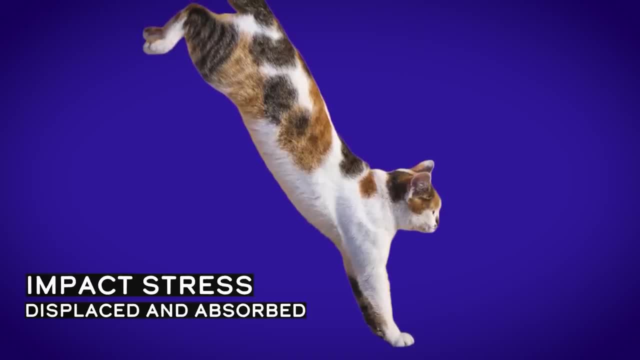 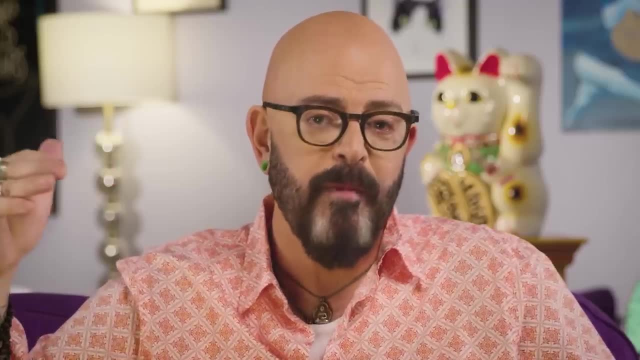 can jump down from great heights. as they hit the ground, then all of that impact is dispersed around their entire system. because they're made for that. cats actually have what's called a writing mechanism. when they fall, they can fall, you know, with their back facing the ground. they find that. 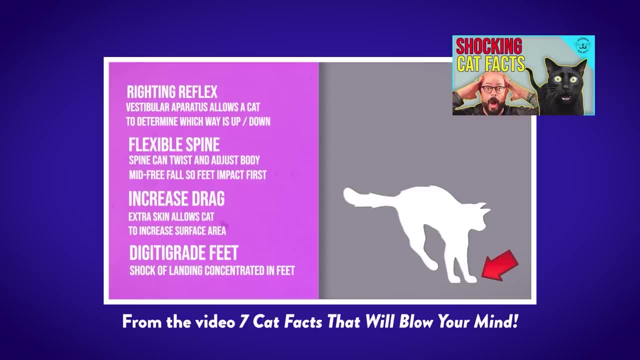 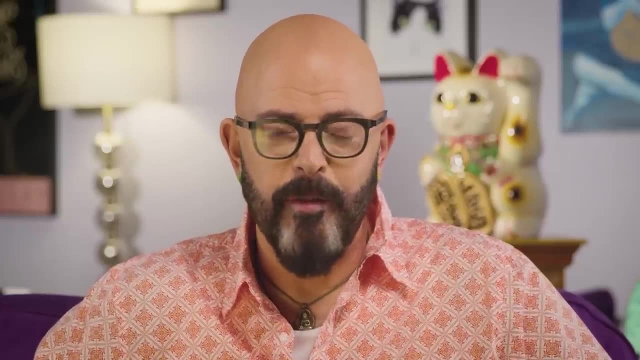 center and they know where the ground is and their whole body turns and they're so much more flexible in this way, and then they know how to land on their feet. dogs just are not built for that. let's talk about how they see the world. both cats and dogs have much better peripheral vision than humans. 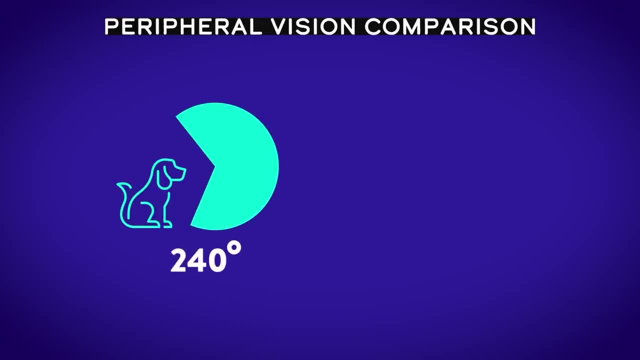 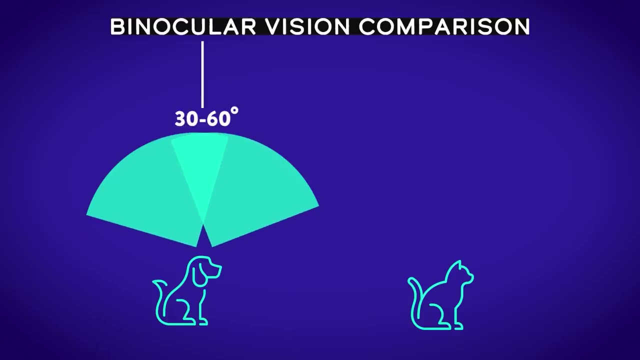 dogs can see about 240 degrees, which is a lot in peripheral vision. cats about 200 degrees, so not as much. now we get a big difference when we start to focus in on a single point of reference or binocular. cats have much better vision than dogs. we're talking 30 to 60 degrees in dogs. 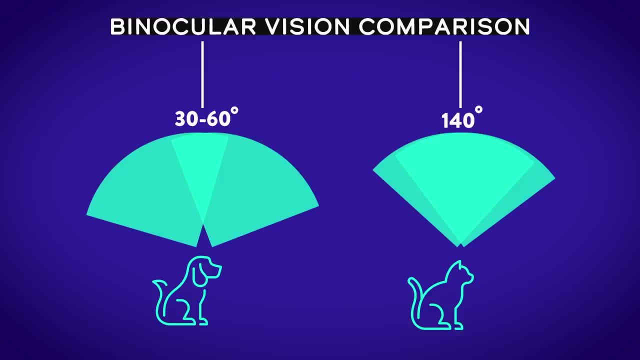 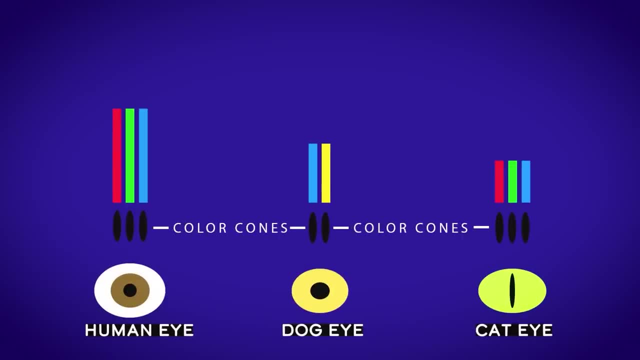 and 40 degrees in cats. so let's talk about colorblind. everyone's always asking: is my dog colorblind? is my cat colorblind dogs? yes, they have limitations in their color perception, very, very much like a human who is colorblind, which is to say, the red, green colorblind cats are just a little. 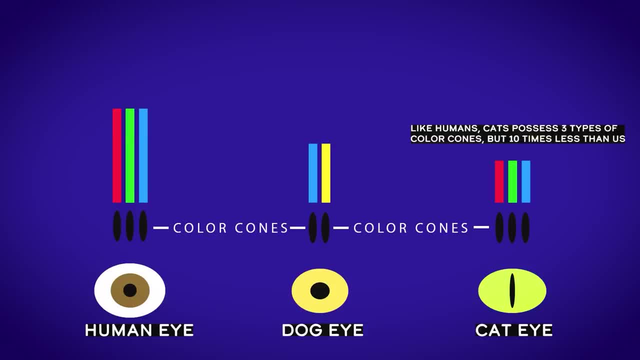 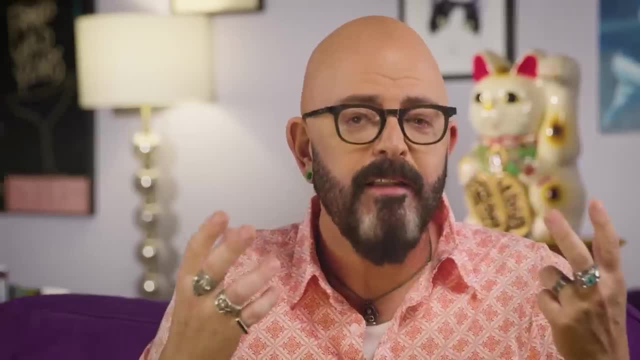 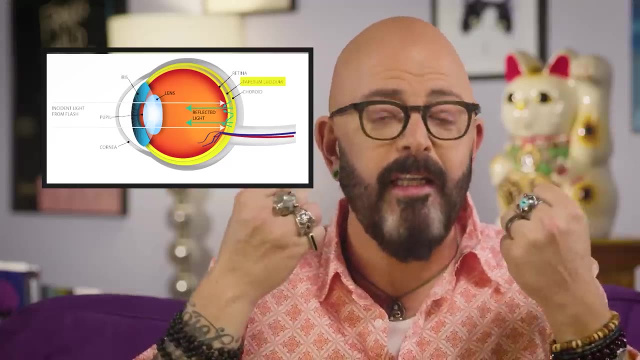 more varied. they, by and large, can see colors better than dogs, and they also see, because of that, contrasting colors better than dogs as well. both cats and dogs have what's called the tapetum lucidum, and that is something in the back of their eyes that allows them to filter in light, even in very low light. cats definitely do more with that. 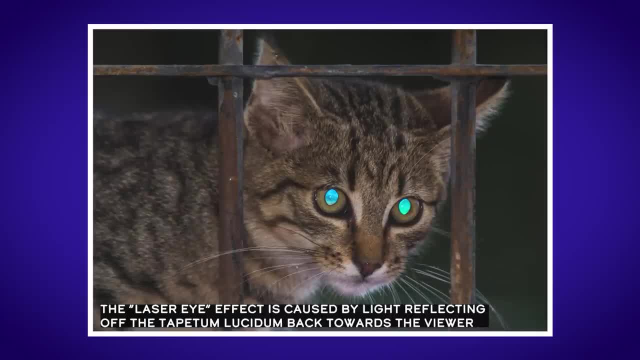 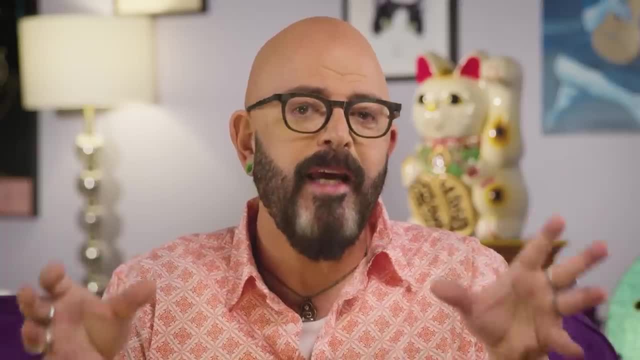 light because they are crepuscular. they hunt in in very low light, whether that's sundown or sun up, because that's when their prey is more available to them. so in a way, yes, cats and dogs can do more with low light, but for instance, with humans and with dogs there are irises when there is. 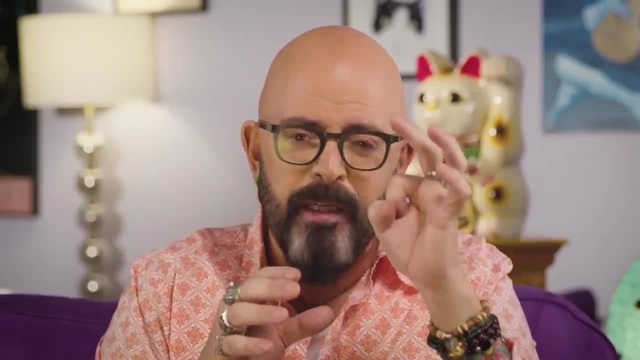 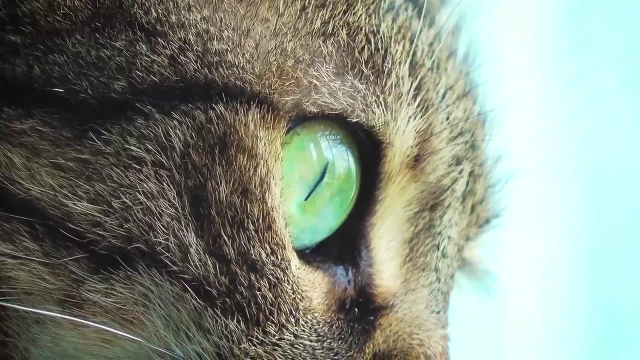 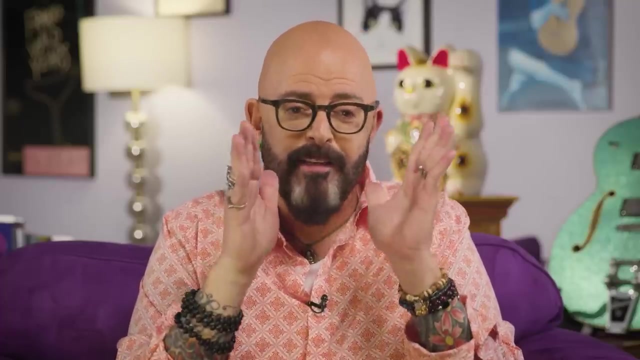 a lot of light it really contracts and into a little bitty pinprick cats. actually it turns into a slit so they can receive more light in there and therefore make a little bit of adjustment. in low light cats can see up into the ultraviolet range, which is to see. I mean it's like you know. 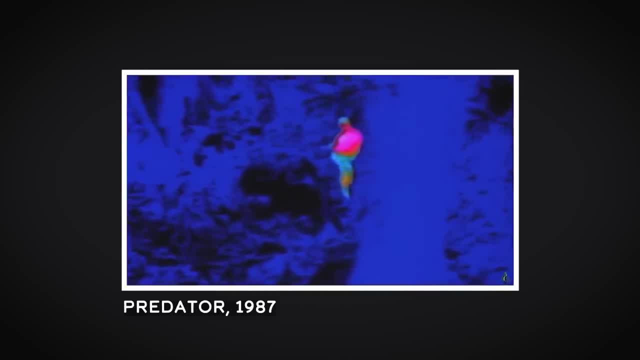 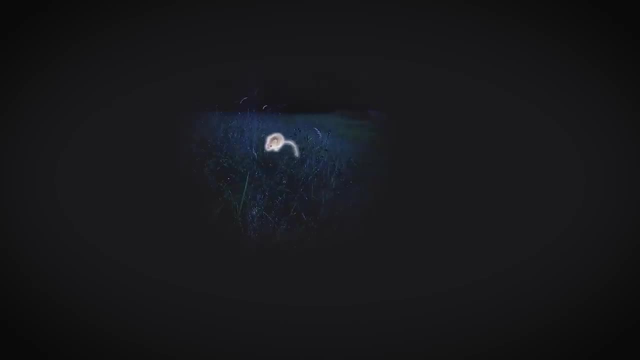 that that movie Predator, where Predator is like. they see those, those figures in in the distance and they don't know what that figure is, but they know that they're there and they know that that's where they're going to eliminate that's, or eliminate their prey. a cat can see way off in the distance, a mouse in grass they can see. 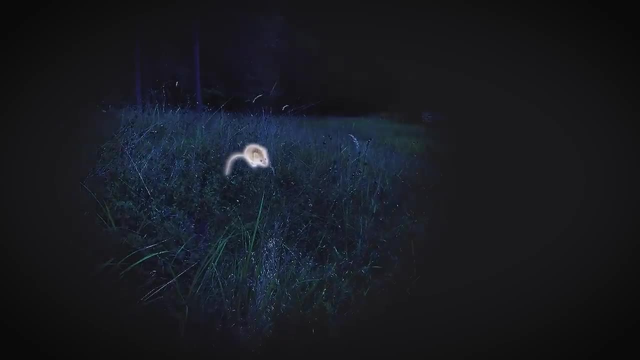 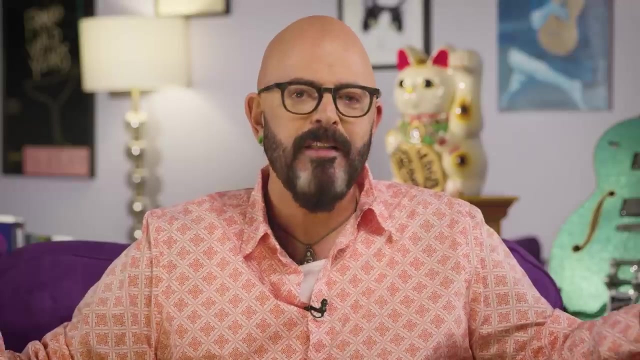 up into that ultraviolet range and actually there are some theories that cats can even see in the infrared range, which is why they can see ghosts. am I getting off topic? I believe I am, but because cats are so dependent on their eyes picking up prey in low light, it really 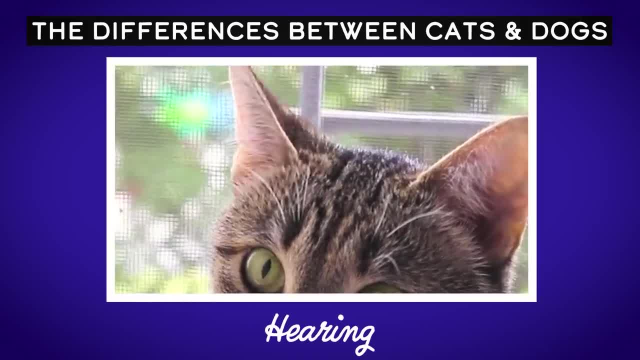 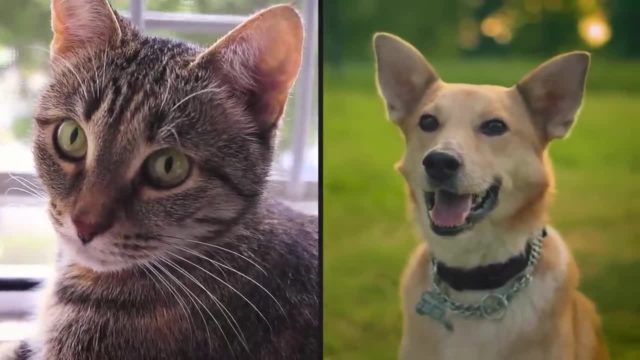 does give them a bit of an advantage. let's talk about hearing dogs and cats both here in a much wider range and with much more acuity, approximately four times better, than humans can. now let's talk about a difference between cats and dogs and a lot of this again. comes from the fact that cats are always hunting or trying to avoid being hunted. cats have nine more muscles in their ears than dogs do. that's because those muscles help to control this radar on the top of a cat's head. their ears can turn almost all the way around so they can focus in. 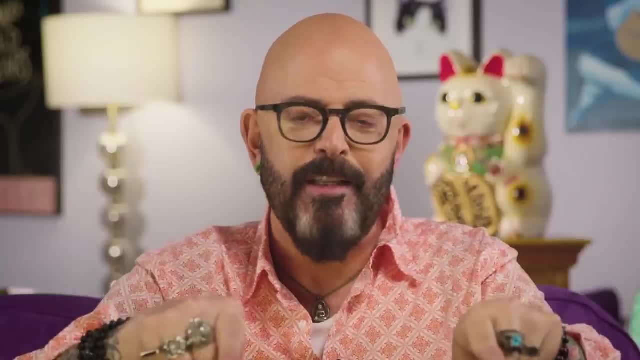 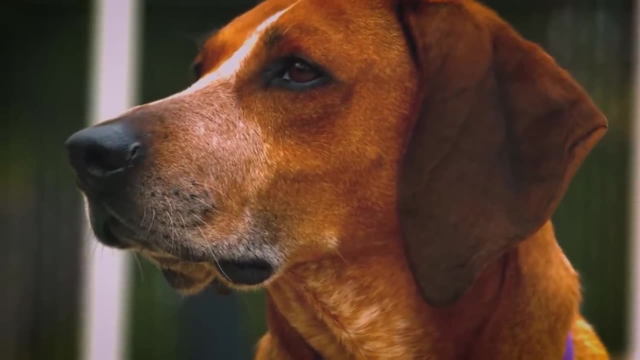 on what they're missing back there and what they're trying to get to up here. so that means that cats have 27 total muscles in their ears alone and dogs only have 18.. cats can also hear in a much higher range than dogs. again, you, 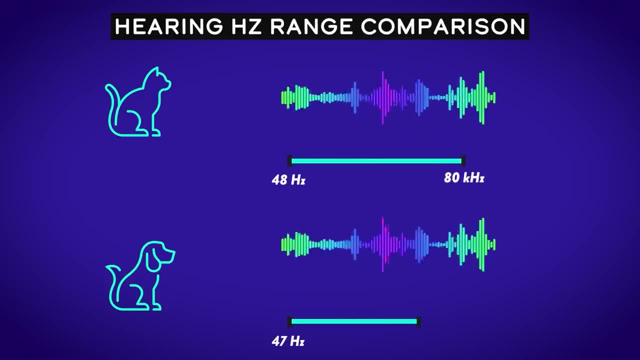 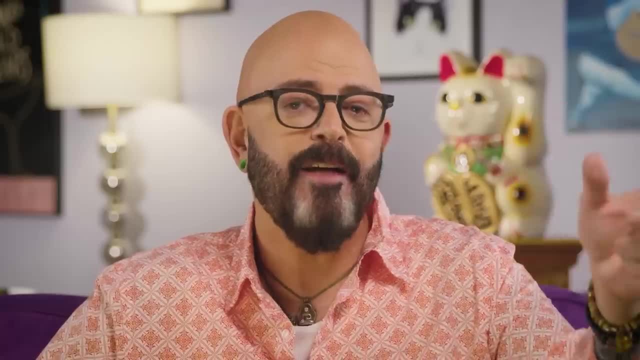 think about what their prey is, whether they're mice or crickets or birds. that's up in that range there. dogs really don't have a use for that. cats can also figure out the distance that sound traveled to get to them. again, hunter be hunted. that's where it all comes from. 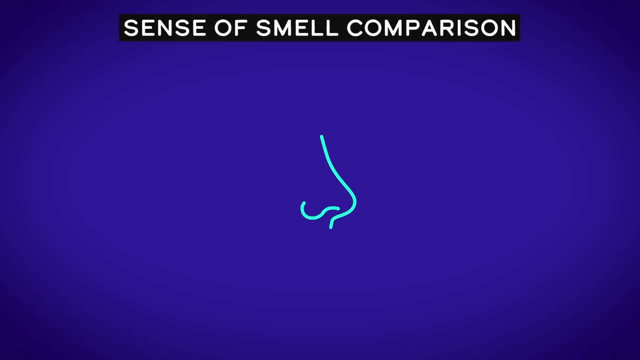 so sense of smell by the numbers, humans have about six million scent receptors in their nostrils. that is a paltry amount compared to both cats and dogs. dogs have on average about 100 million, but it can get up to 300 million. cats have about 200 million scent receptors in their nose. so because of these, 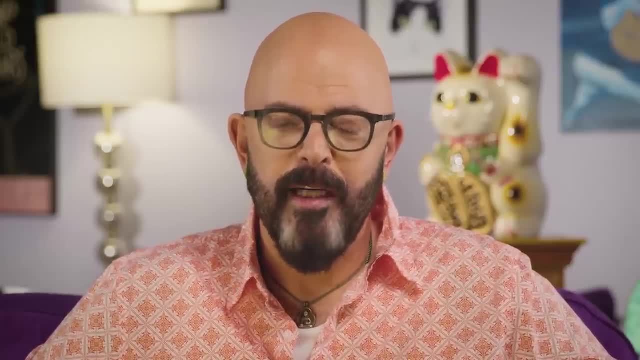 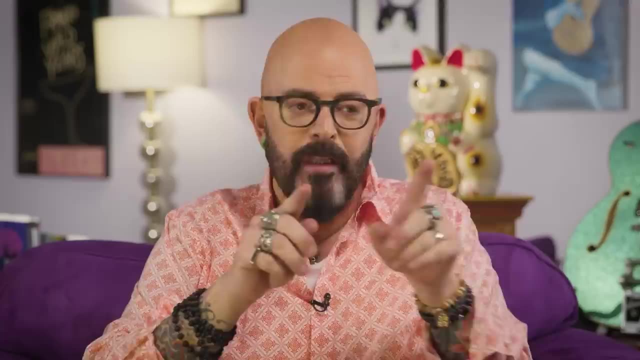 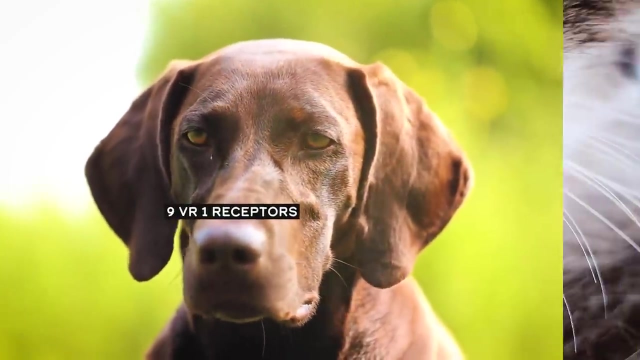 numbers. historically, it was thought that dogs just had a better sense of smell, but the fact is, as we start to break down the types of receptors in their nose, there's this one type of receptor that's responsible for distinguishing between sense, that's the v1r receptor. humans only have two of them, dogs have nine, cats have 30, because, again, it's so.